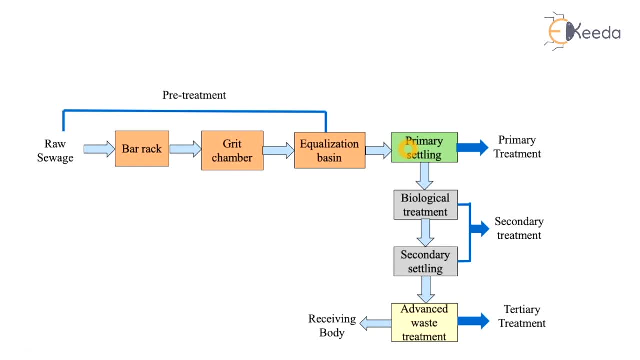 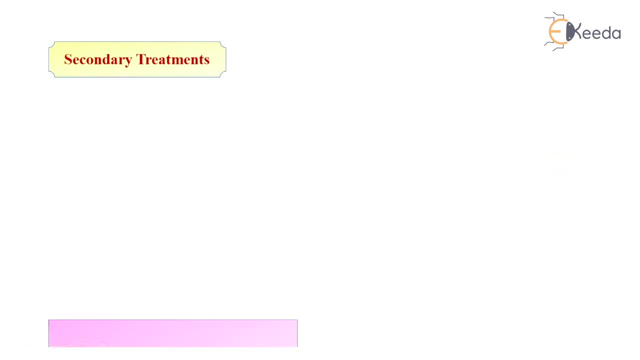 Then we remove the settleable organic matter and then we move for the secondary treatment. There are various methods which can be adopted as a secondary treatment. The basic classification is of two types. First is attached growth system and second one is suspended growth system. 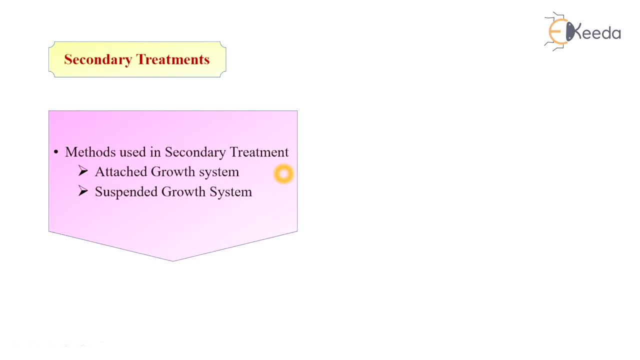 So in attached growth system the biomass is there, attached to the media, Then the sewage passes through this media and clarification happens. So whatever, the typical examples in this process are the intermediate: sand filter, trickling filter, rotating biological contactor, etc. 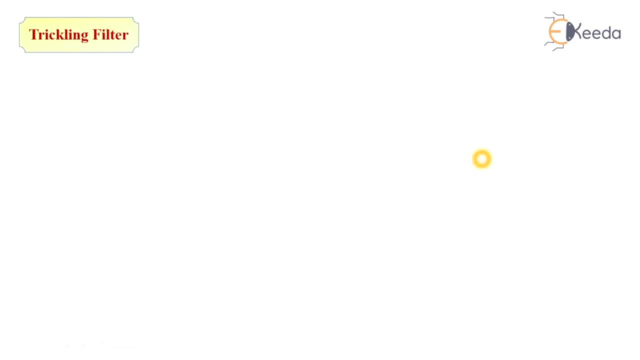 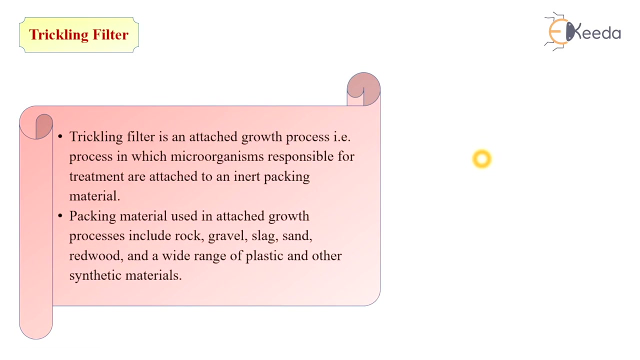 So let's, we will see one by one. So first is trickling filter. Trickling filter for biological filtration of sewage, The conventional trickling filter and their improved form known as high rate trickling filter, are now almost universally adopted for giving a secondary treatment to sewage. 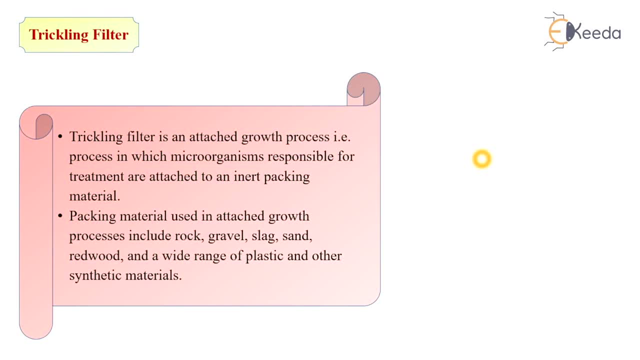 These filters, also called as percolating filters or sprinkling filters, consist of a tank of coarser filtering media over which the sewage is allowed to sprinkle or trickle down by means of spray nozzles or rotary distributors. The percolating sewage is collected at the bottom of tank through a well designed under drainage system. 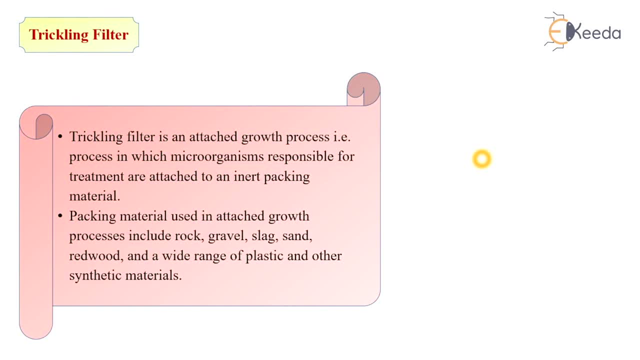 The purification of the sewage is brought about mainly by the aerobic bacteria, which forms a bacterial film around the particles of filtering media. The action due to the mechanical straining of the filtering media is much less In order to ensure the large scale growth of aerobic bacteria. 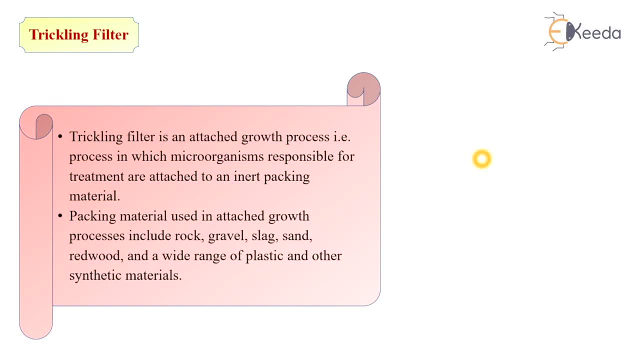 sufficient quantity of oxygen is supplied by providing a suitable ventilation facility in the body of filter. The influent obtained from the filter must be taken to the secondary sedimentation tank for settling out the organic matter oxidized while passing down the filter. The sewage influent entering to the filter must be given. 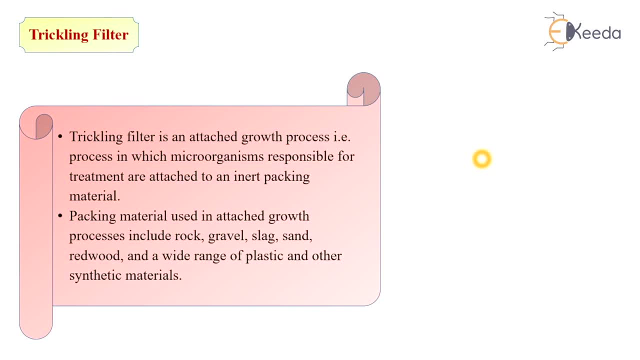 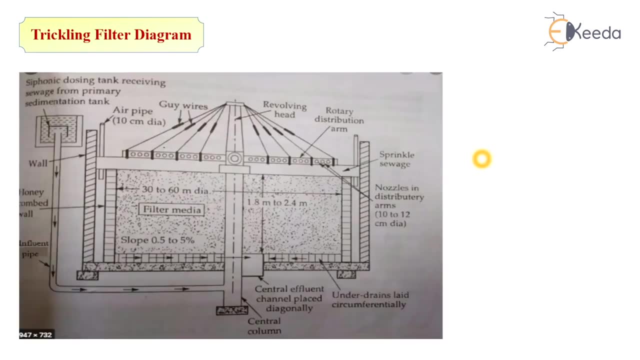 pre-treatment, including screening and primary sedimentation. So we will see the construction and operation of trickling filter. Trickling filter tank are generally constructed above the ground. They may either be rectangular or, more generally, circular. The rectangular filters are provided with network of pipes. 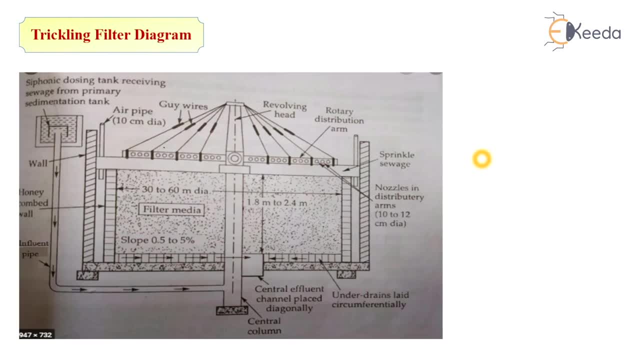 having fixed nozzles which spray the incoming sewage into the air, which then falls over the bed of filter under gravity. The circular filter tank, as you can show in this figure, on the other hand, are provided with rotary distributors. So, as you can see in this figure, so these are the rotary distributors. 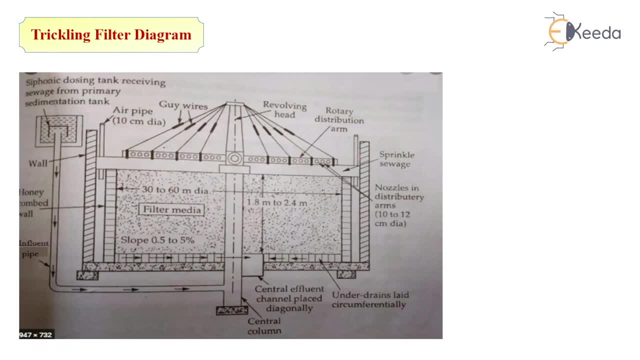 having a number of distributing arcs. These are total 8 number of distributing arcs. These distributors rotate around the central support, either by the electric motor or, more generally, by the force of reaction. So this is the central support or vertical column. Such self-propelled reaction type of distributors are nowadays preferred as used. 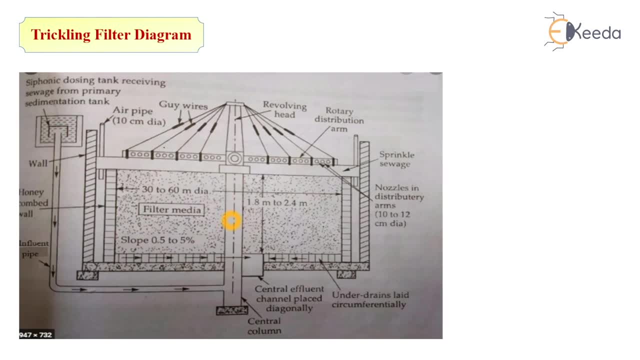 The advantage of having two or more arms is not only to get the reaction sufficient to rotate the entire mechanism, but is also to pass the fluctuating demand by taking low flow in two arms and the remaining two arms coming into the operation only at the time of higher flow. 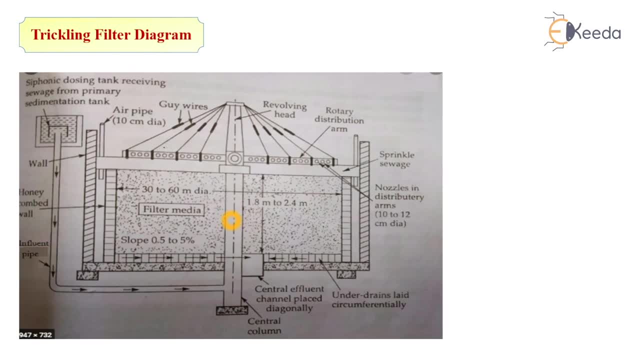 With the rotary distributor, the application of sewage to the filter is practically continuous, Whereas with spray nozzles the filter is dosed for 3 to 5 minutes and then then rested for 5 to 10 minutes before the next application. 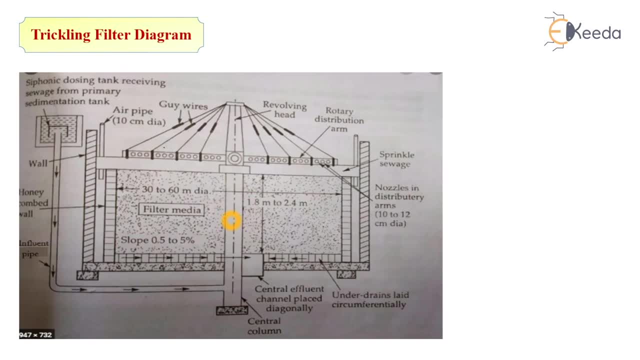 The filtering media, as you can see in this figure. So these are the filtering media, as pointed out earlier, consist of coarser material like cubically broken stones or slag, free from dust and small pieces. The size of the material used may vary between 25 mm to 75 mm. 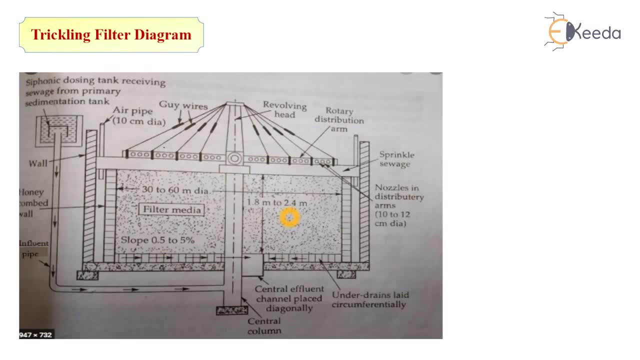 The filtering material should be washed before it is placed in position. The quality of the stone used should be such as not to be easily affected by acidic sewage, and should be sufficiently hard. The depth of the filtering media may vary between 2 to 3 meters. 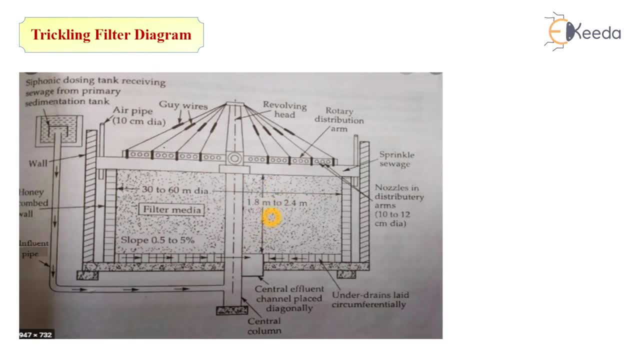 So this depth is between 2 to 3 meters. The filtering material may be placed in layer with coarser stone used near the bottom and finer material towards the top. The walls of filter tank are made honeycomb or otherwise provided with openings for circulation of air. 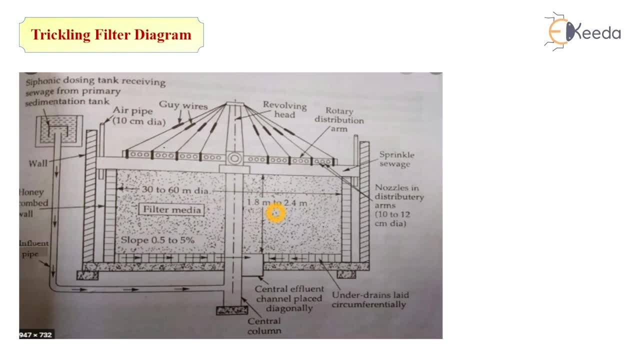 A satisfactory ventilation is achieved Then properly designed under drainage system. as you can see in this figure at its bottom, This is the under drainage system provided to the filter bed. Beside ensuring the satisfactory drainage, such a drains will also ensure the satisfactory ventilation and aeration of the filter bed. 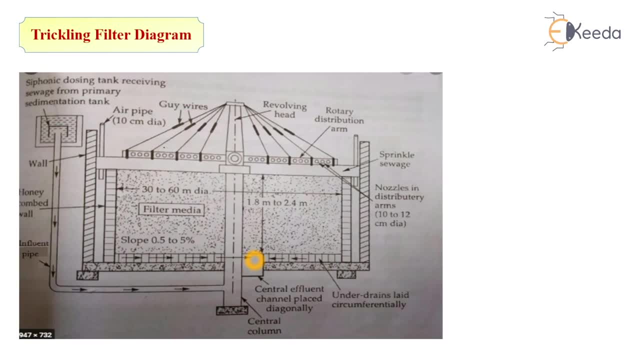 The blocks have top openings of such a size that the stone can be placed directly on them. These blocks are laid on the reinforced concrete floor towards the main effluent rectangular channel. This main effluent channel may be provided adjoining the central column of the distributor, as shown in figure. 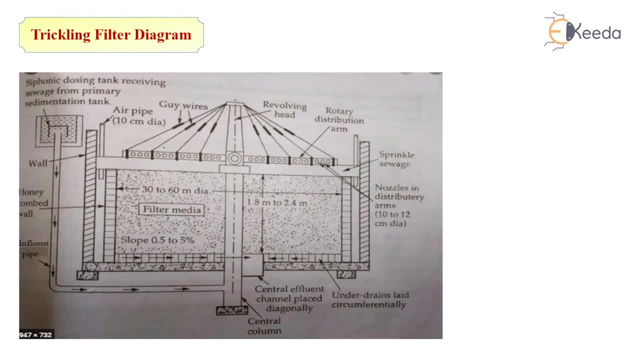 So this is the central effluent channel placed diagonally. The slope of the channel should be sufficient to enter the filter bed. So this is the central effluent channel placed diagonally. The depth and the width of this central channel should be such that the maximum flow is carried below the level of under drainage. 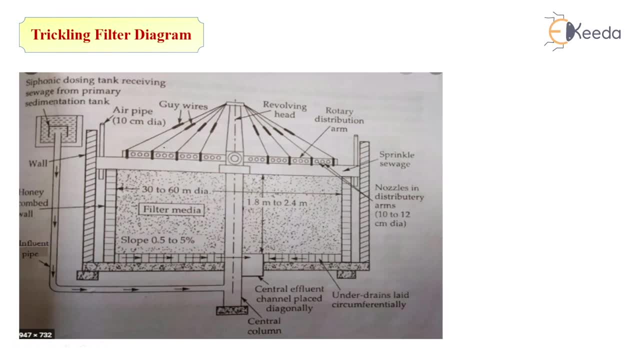 So this is the typical diagram of trickling filter So, which contains a circular or rectangular tank, a central vertical support, the distributory arms, distributory chamber and distributory arms, the nozzles through the nozzles To which the sewage is sprinkled through this filter media. 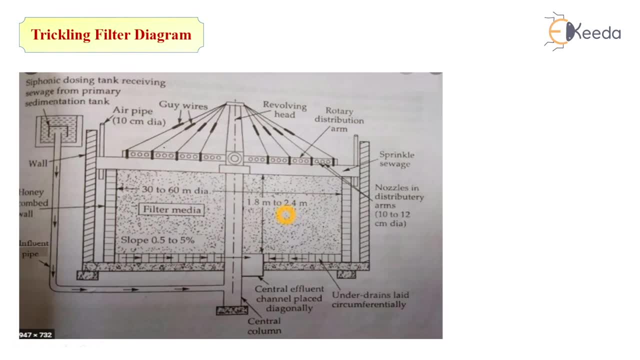 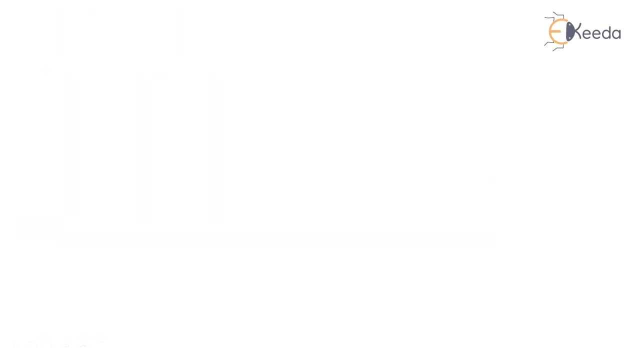 Filter media in the coarser size, placed in layers. The depth of this tank should be 2 to 3 meters, Slope should be provided, Under drainage system should be provided And central effluent channel should be provided. So the process description of trickling filter is. 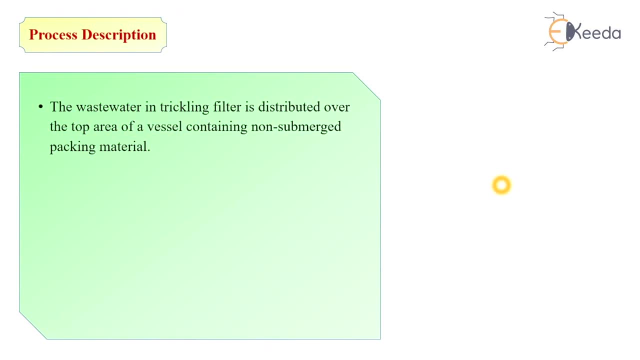 First, the waste water in trickling filter is distributed. Water in trickling filter is distributed over the top area of vessel containing non submerged packaging material. The air circulation in the void space by earth, either natural draft or blowers, provided oxygen for the microorganism growing as an attached biofilm. 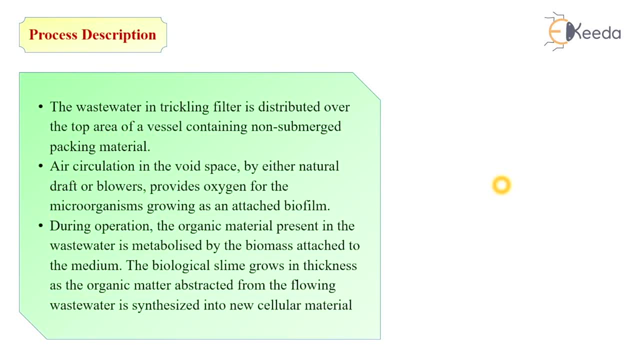 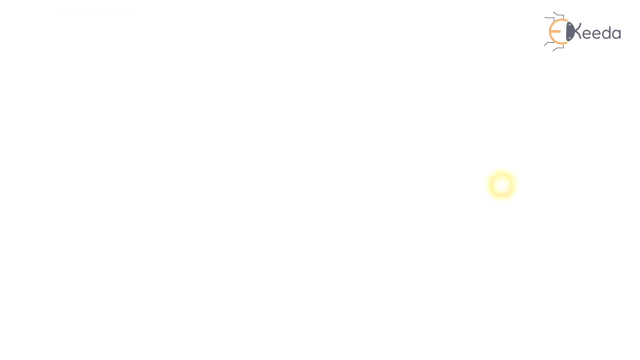 During the operation the organic material present in the waste water is metabolized by the biomass attached to the medium. The biological sling growth in thickness as the organic matter abstract from the flowing waste water is synthesized into the new cellular material. Then the thickness of the aerobic layer is limited by the depth of penetration of oxygen into the microbial layer. 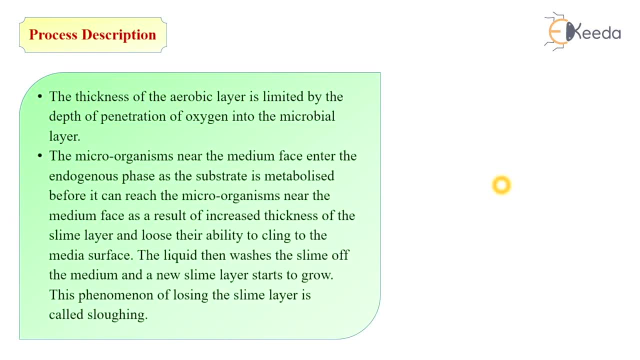 The microorganism near the medium phase enter the endogenous phase, that is, anaerobic phase, As the substrate is metabolized Before it can reach to the microorganism near the medium phase as a result of increased thickness of the slime layer, 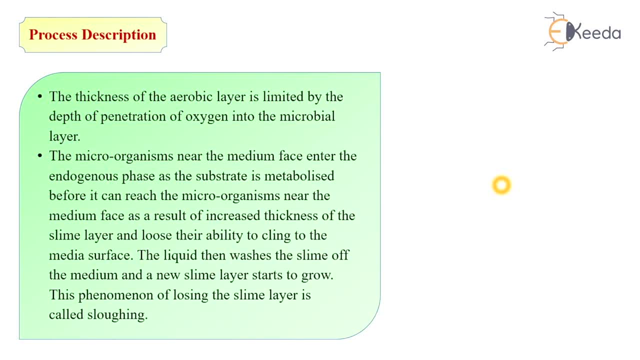 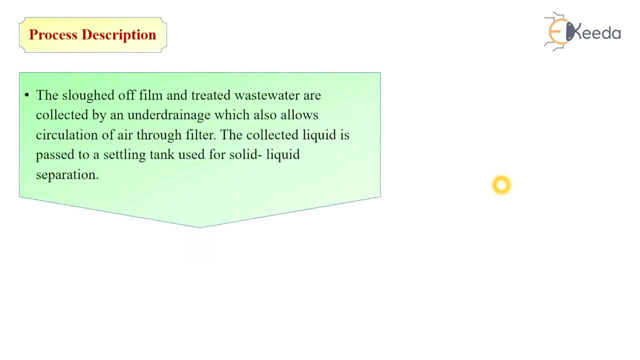 And those their ability to clean to the media surface. The liquid then wash the sling of the medium and the new sling layer starts to grow. This phenomenon of losing the slime layer is called as slogging. The slog of film and treated waste water are collected by the sling layer. 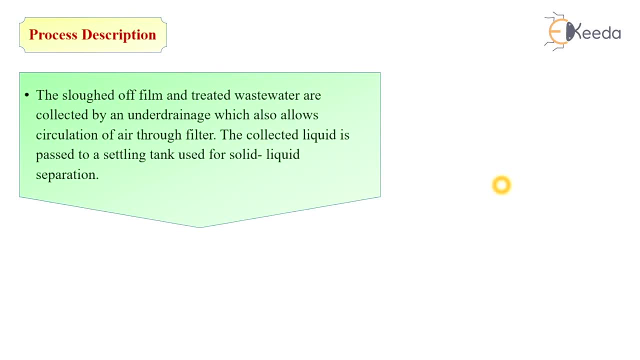 And are collected by the under drainage, which also allow circulation of air through filter. The collected liquid is passed to the settling tank used for the solid liquid separation. So, as I discuss the mechanism of trickling filter As the sewage passes through this filter bed, 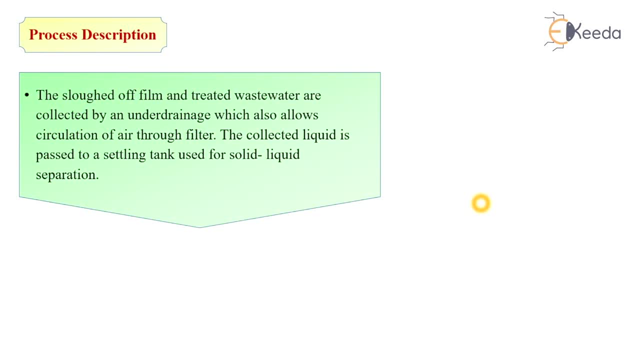 It comes in contact with filter media. On this filter media, a biofilm is formed In form of slime layer. So the formation of this biofilm is called as slime layer. It consists of biomass in terms of bacteria, protozoa and the cell of microorganism. 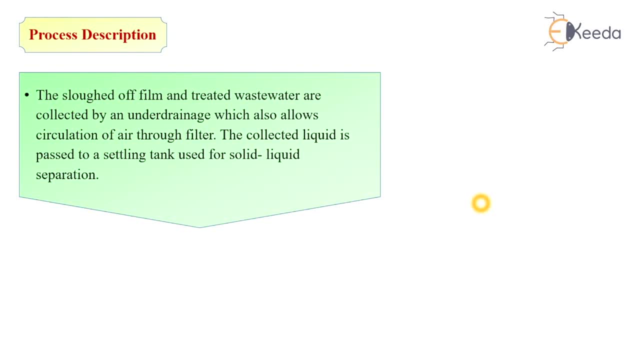 So as the sewage passes through this filter bed, It will comes in contact with slime layer, And organic matter present in sewage are act as a food for this slime layer or microorganism, So the organic matter are absorbed on this surface of the media. 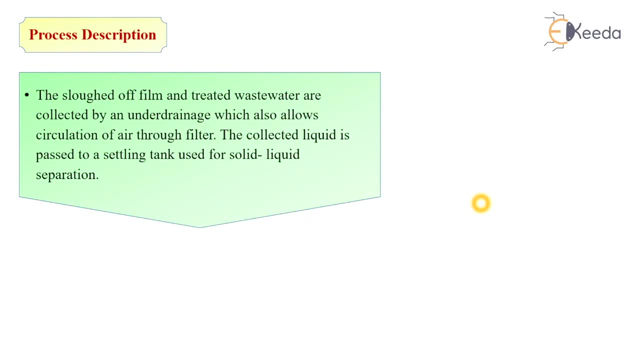 The microorganism or bacteria present in the slime layer Which will oxidize the organic matter in stable form. So this is the surface of filter material. So just you imagine a circular stone And around this surface of filter material, On this surface the slime layer is formed. 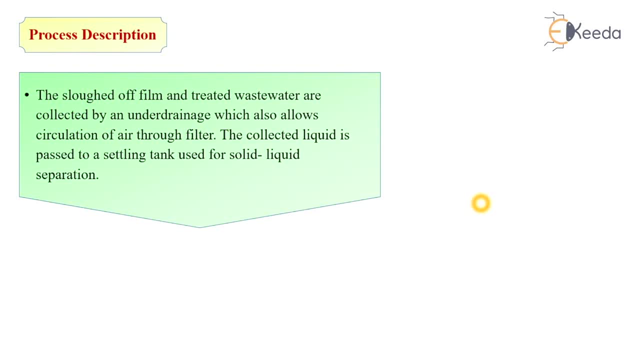 On the top of this slime layer a proper oxygen supply is there. So in this whole zone The biomass is present And the upper part of this slime layer. That depth is between 1 meter, So this upper part is in aerobic condition. 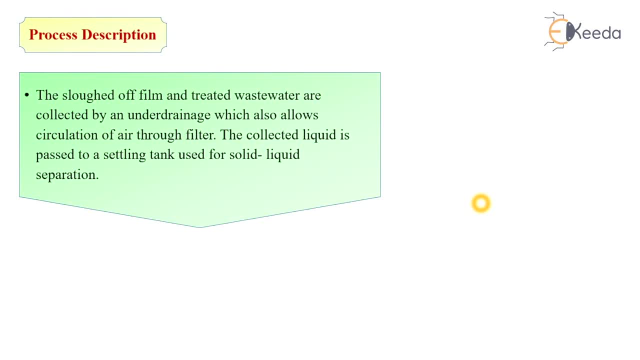 And the part from that. the rest of the part is in anaerobic or endogenous phase Or anaerobic condition, Because the oxygen does not reach up to this part. So the organic matter comes in this slime layer. More food is provided for microorganism. 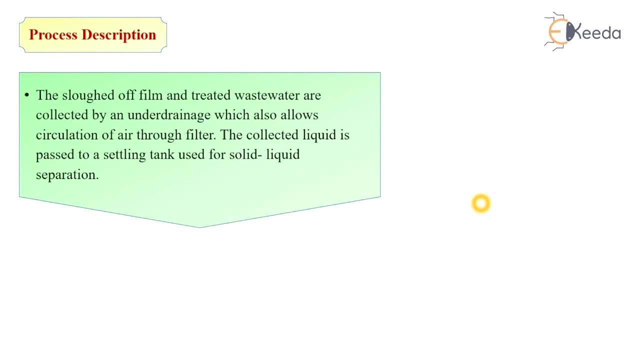 There is a ample supply of oxygen And ample supply of organic matter as a food. The bacteria present in the blue zone. That is rapid growth phase. So the thickness of slime layer will be increasing. So the top portion of this layer is called as blue zone. 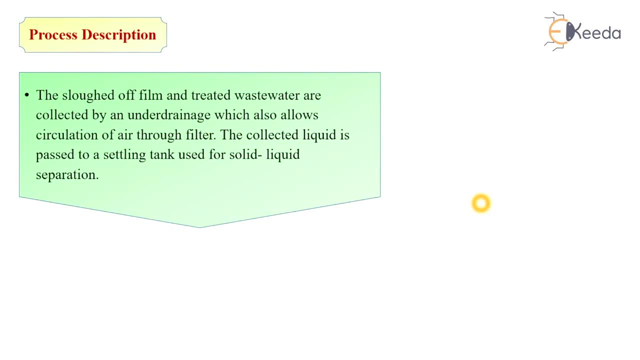 Due to increase of thickness, The lower part of the slime layer phase. The deficiency of oxygen is there And the aerobic condition exist in the lower part, So not getting organic matter as a food. So they enter in the endogenous phase or anaerobic phase. 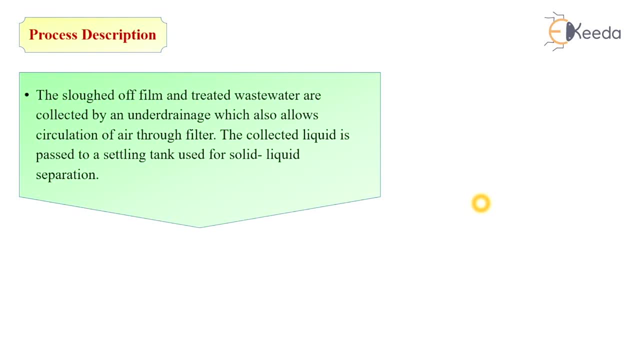 So they use their own cell material for their existence? So they do not. So they lost their capacity to hold. So that slime layer loses its capacity And it will be automatically fall down. So the washing of that slime layer will happen. That mechanism or phenomenon is called as slogging. 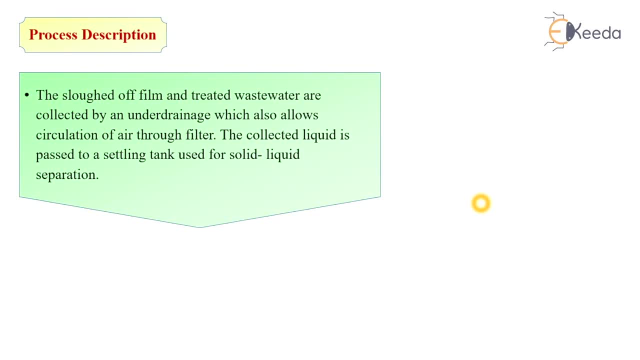 So there are different technical terms We are used in this mechanism of trickling filter. The first is organic matter, Then the bacteria or microorganism, Then the slime layer or biomass or biofilm, And then the slogging of slime layer. 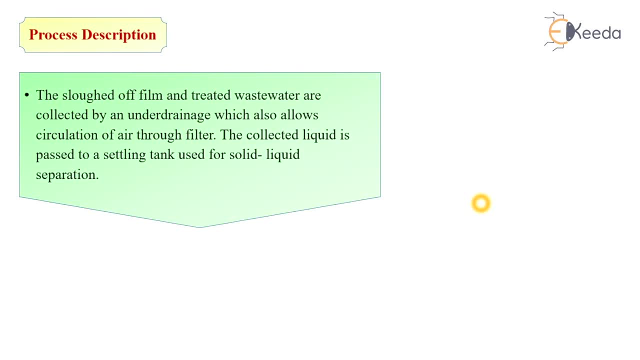 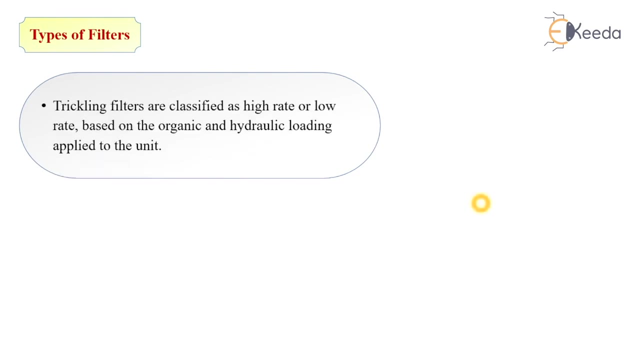 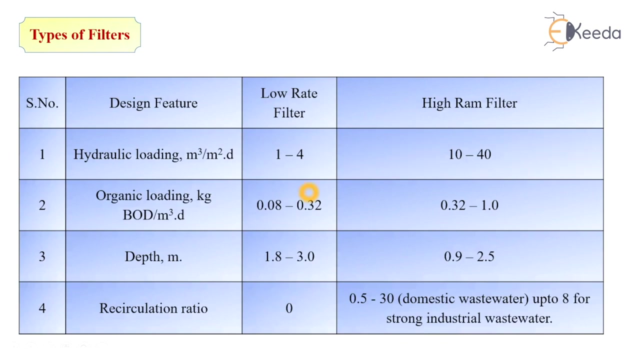 Or washing of this slime layer. So the types of trickling filter. The trickling filters can be broadly classified into The conventional trickling filter And high rate trickling filter. That is conventional is the low rate trickling filter And high rate trickling filter. 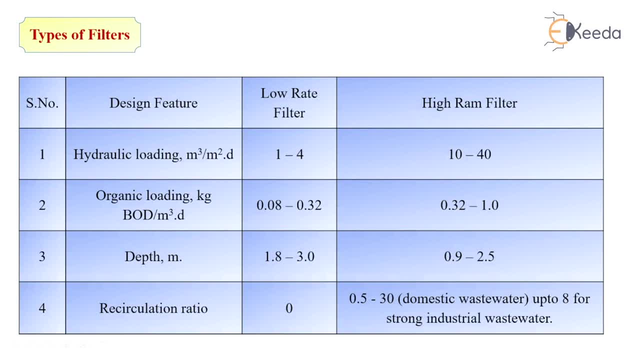 So here are some, A comparison of these two types, Depending on its design parameters, That is, depending on its hydraulic loading, Organic loading Depth And recirculation ratio. So all these parameters, or definition of these parameters, That we will see in next part in detail, 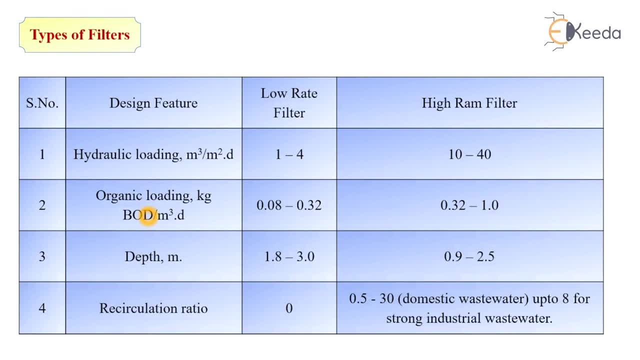 While we are solving the problems on trickling filter. So here you just remember the figures Or the values of this both. So hydraulic loading rate in terms of meter cube Per meter square per day For low rate trickling filter is 1 to 4.. 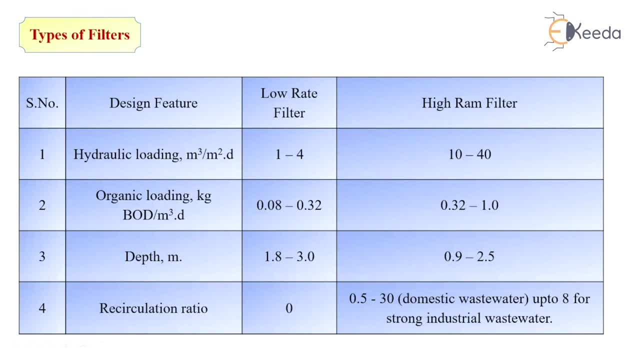 And for high rate trickling filter is 10 to 40.. The organic loading in terms of kg, That is, BOD per meter cube per day, For low rate trickling filter is 0.08 to 0.32.. And for high rate trickling filter is 0.32 to 1.. 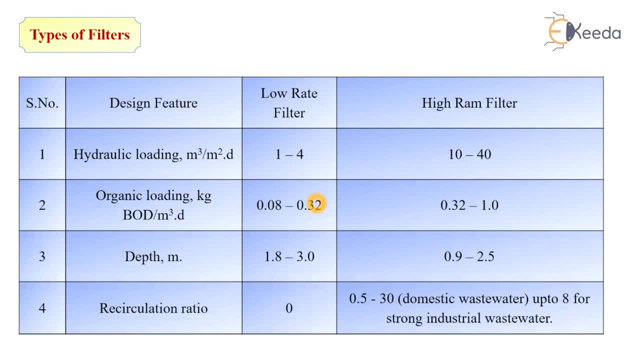 The depth of conventional trickling filter is maximum, That is, 1.8 to 3 meter, And for the high rate trickling filter is 0.9 to 2.5 meter, And the recirculation ratio for the low rate trickling filter is 0.. 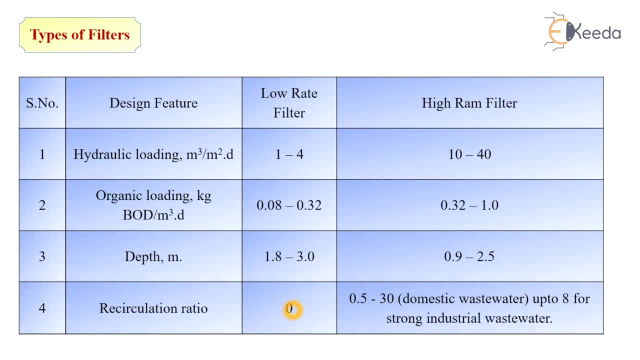 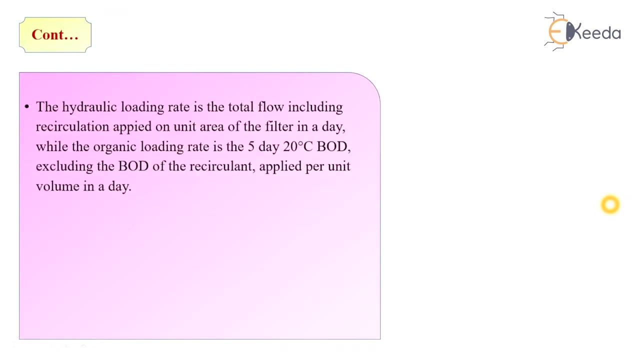 So there should not be provided any recirculation. And for the high rate trickling filter, The 0.5 to 30 up to 8.. For strong industrial waste motor The recirculation will be provided. So the hydraulic loading rate. 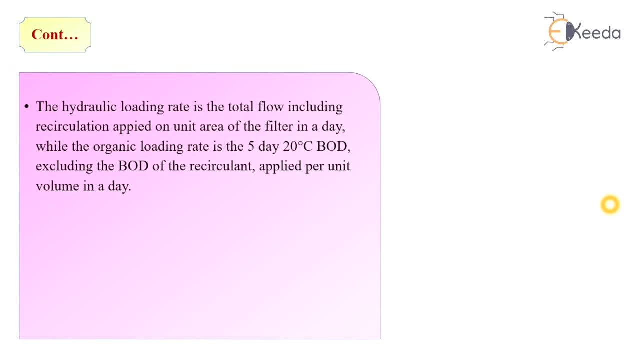 Is the total flow, Including the recirculation, Applied on the unit area of the filter, in a day, The total flow of sewage. So it is nothing but the discharge of sewage, Or sewage flow or sewage discharge, While the organic loading rate 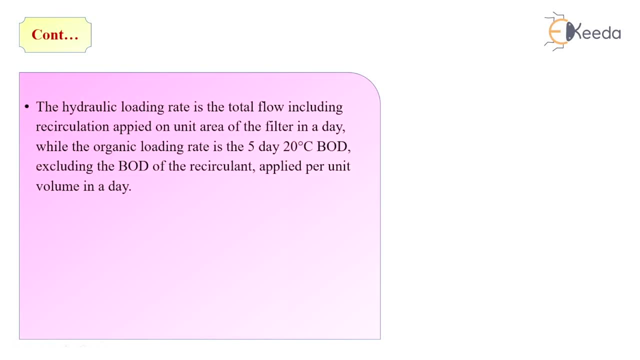 Is the 5 days at 20 degree centigrade, The BOD value, Excluding the BOD of the recirculant, Applied per unit volume in a day. So hydraulic loading rate. So hydraulic loading is nothing but the sewage flow. 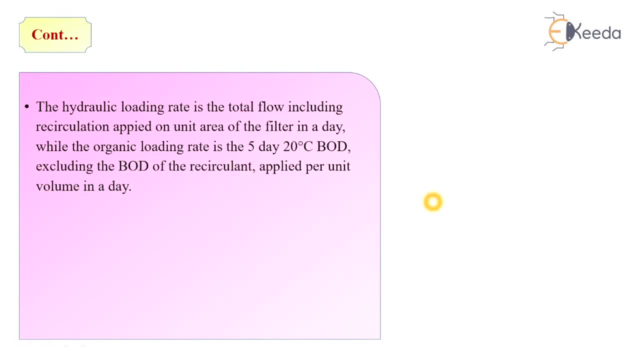 And organic loading is nothing but the BOD value. Recirculation is generally not adopted In low rate trickling filter. As we have seen in previous slide, A well operated low rate trickling filter Is combination with the secondary settling tank. 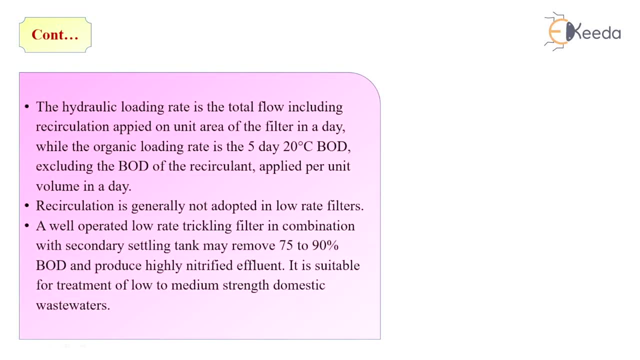 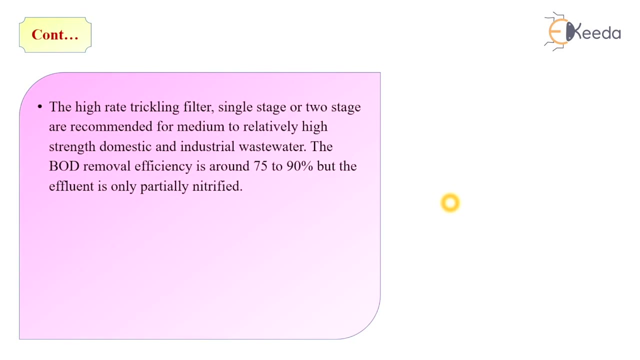 May remove 75 to 90% of BOD And produced a highly neutrified effluent. It is suitable for treatment Of low to medium strength domestic wastewater. The high rate trickling filter, Single stage or two stage, are recommended For medium to relatively high strength. 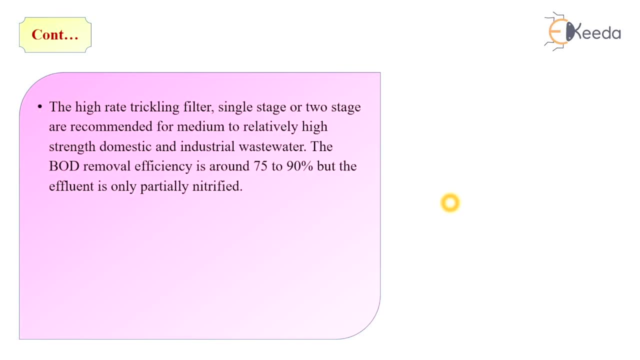 Domestic and industrial wastewater. The BOD removed efficiency In high rate trickling filter Is around 75 to 90%, But the effluent is only partially neutrified. Single stage unit consists of: Primary settling tank Filter, Secondary sedimentation tank, 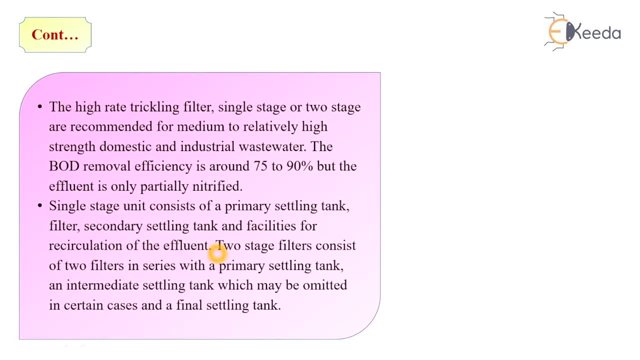 And facilities for recirculation of the effluent Where in two stage filter Consist of two filters in a series, With a primary settling tank And an intermediate settling tank, Which may be omitted in certain cases, And the final settling tank. 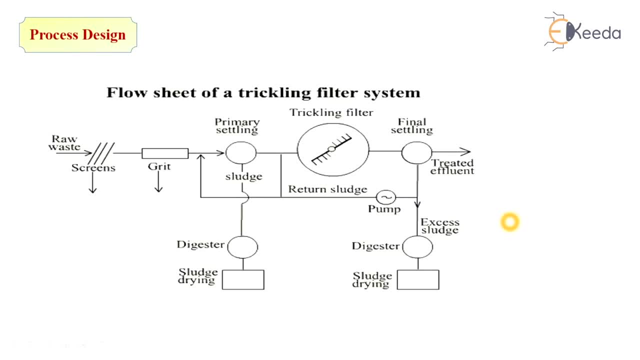 So as you can see in this Flow sheet of trickling filter, So same flow sheet We are see in The previous module, That is, in primary treatment plant. So In primary treatment We are providing the screening And grid chamber. 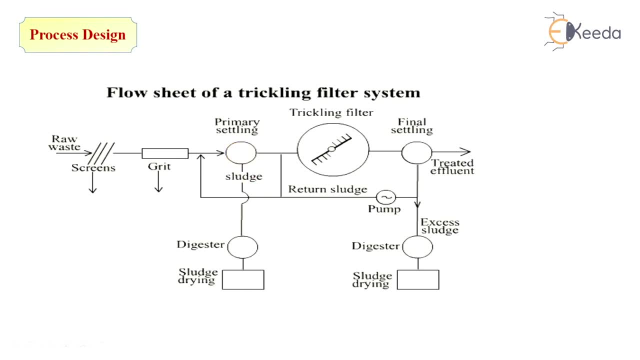 And primary sedimentation tank And in secondary treatment We are providing trickling filters And final set Final settlement tank Or final settling tank. Then This collected or settled sludge Can be passed through this digester To the digester. 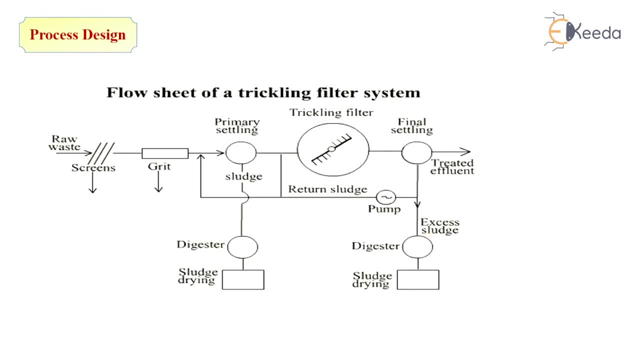 And some part of the sludge Should be recirculate To this trickling filter And then, Ultimately, the sludge Is passed to the sludge drying beds And treated effluent is going for the further treatment, For the or for the tertiary treatment. 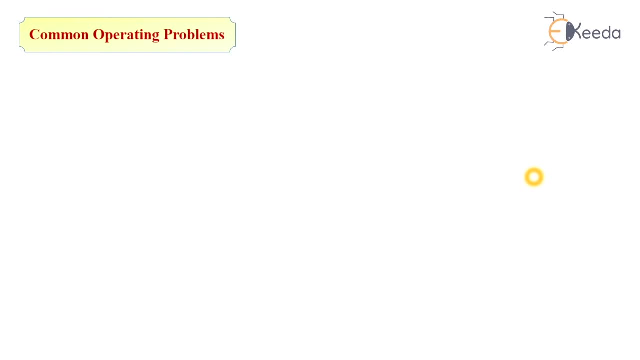 So Next is the common operating problems Facing in trickling filter. First is filter ponding. So what is filter ponding? If the voids in the media Get plug, Flow can collect on the surface In ponds- Excessive slogging. 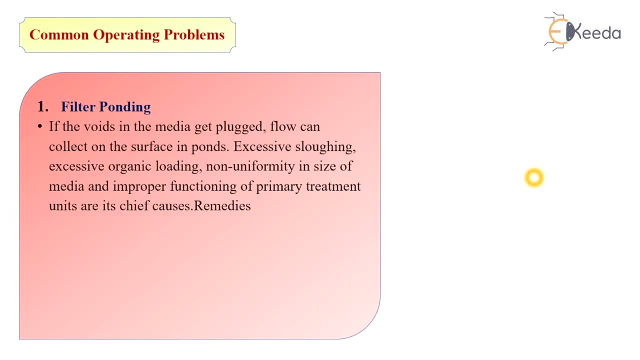 Excessive organic loading, Non-uniformity in size of media And improper functioning Of primary treatment units Are its causes. Some of the causes, So remedy Remedies should be: Wash the filter surface With the stream of water. 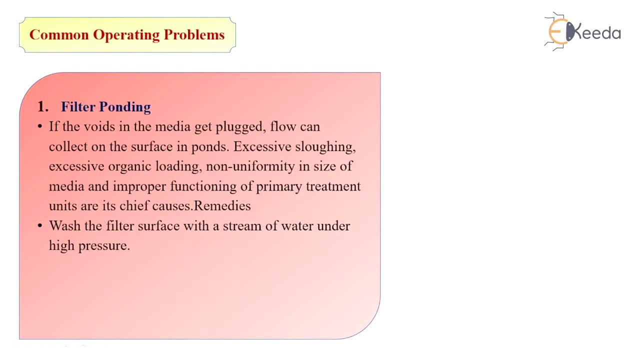 Under the high pressure. So one of the operational problems Facing in trickling filter Is filter ponding. So reasons or causes Of this filtering Pondings are Excessive organic loading, Non-uniformity of size, The excessive slogging. 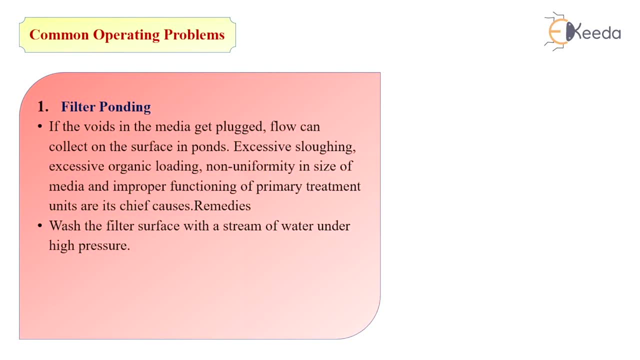 Etc. And in terms of remedies, We are washing this With the help Of the filter, And then We are going to Wash the filter With the help Of the filter, And then We are going to Wash the filter. 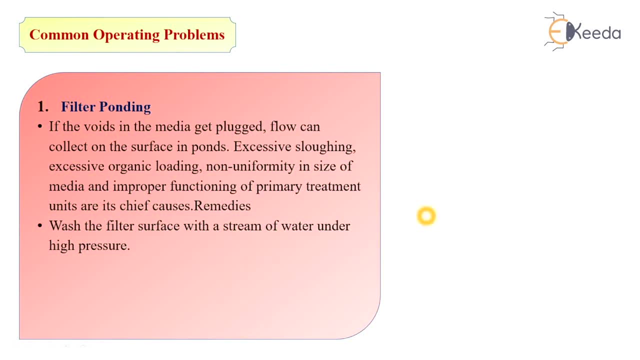 With the help Of the filter. And then We are washing this Filter media With the high pressure Of water, Dose the filter With heavy applications Of chlorine Or take the filter Out of service For the period. 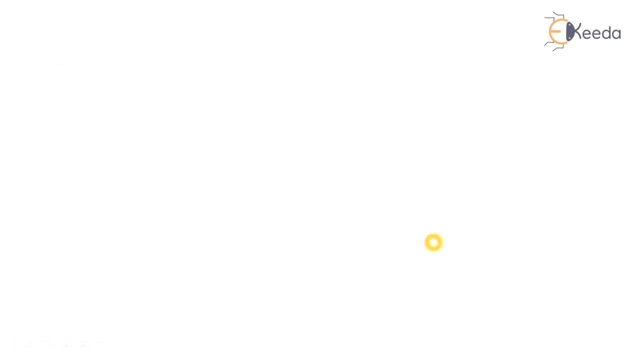 Of one day Or longer To allow it To dry out. So next Problem facing In filter- Trickling filter- Is filter flies- Primary nuisance Insects- Tiny Gnat-sized Filter flies. So this is. 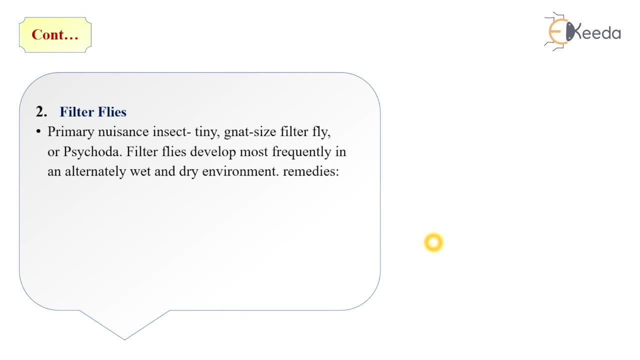 Gnat-sized Filter fly Or Psychoda Filter flies Develop Most frequently In An alternate Wet and dry Environment. So remedies For that Are Dose filter Continuously, Not Intermittently. 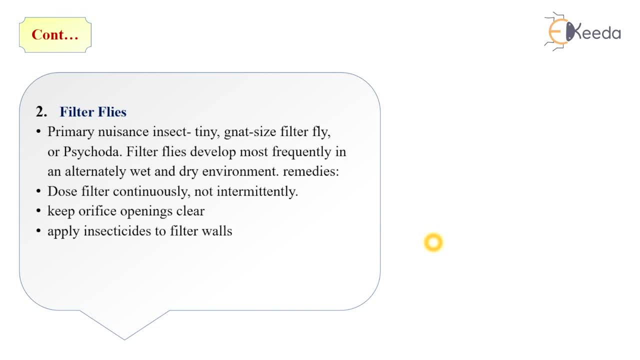 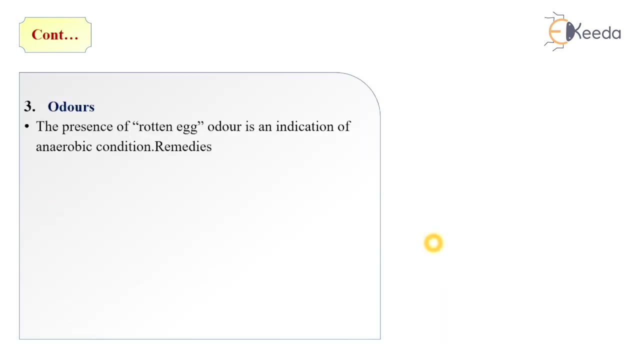 Keep Orifice Opening Clear, Apply Insecticides To the filter Wall, Dose filter With chlorine And keep Weeds In Water. Next Problem Is Of Order: The Presence. 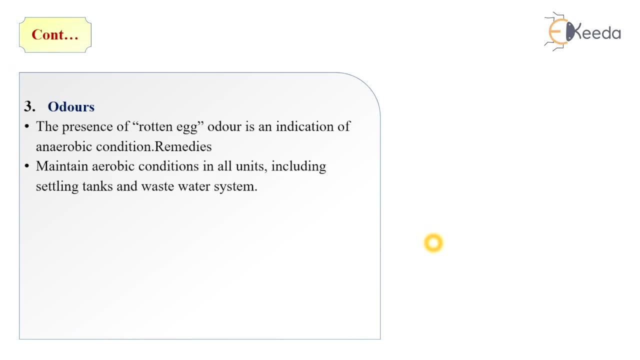 Of Rotten Egg Order Is An Indication Of Unaerobic Condition. So Remedies For That To Maintain The Aerobic Conditions In The Efficiency Of. 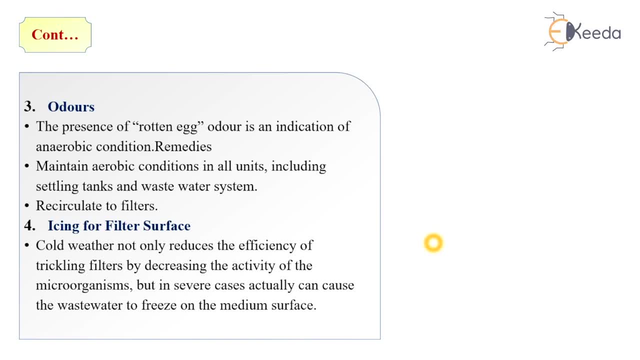 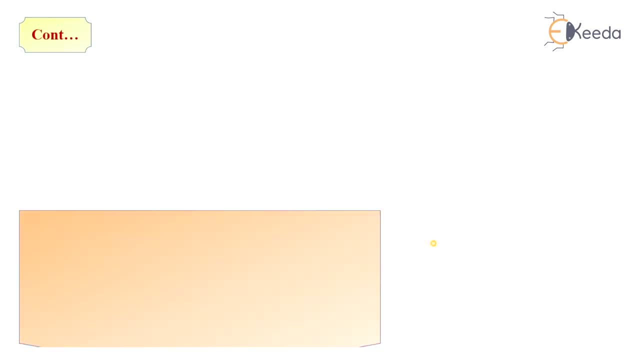 Trickling Filter By Decreasing The Activity Of The Micro Organism, But In Sea Work Cases Actually Can Cause The Wastewater To Freeze On. 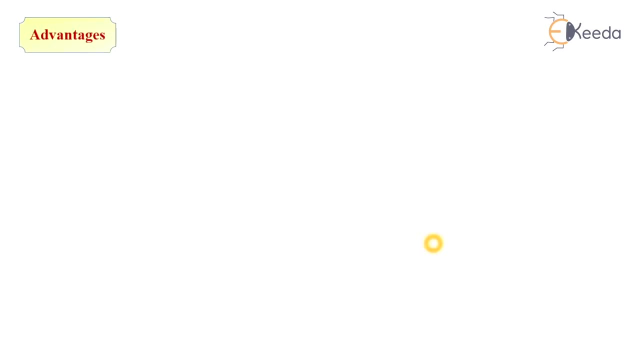 The Medium Surface. So There Are Some Disadvantages And Disadvantages Of This Trickling Filter. So Advantages Are: The Effluent Obtained Is Highly. 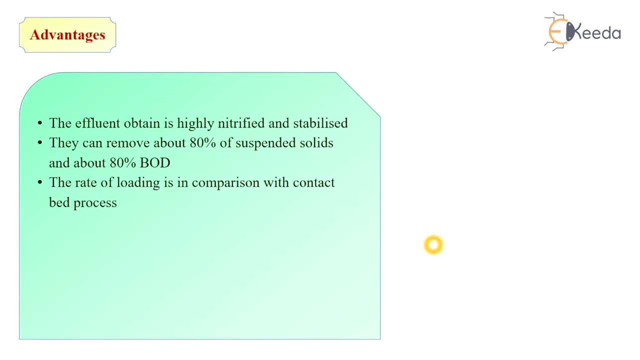 Nutrified And Stabilized. They Can Remove About 80% Of Suspended Solid. They Are Self Cleansing. The Mechanical Wear And Tear Is Less. 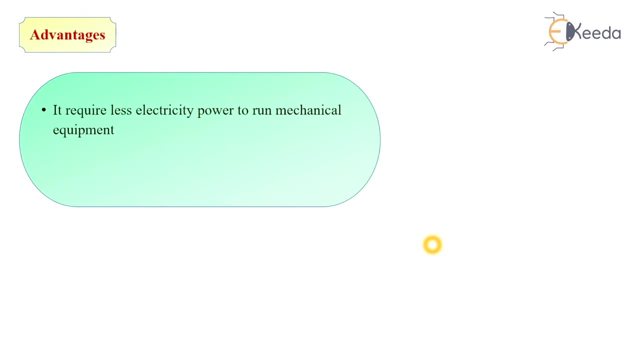 As It Contains Less Mechanical Equipment, It Required Less Electricity Power To Run Mechanical Equipment And The Moisture High Capital Cost The Loss Of Head. 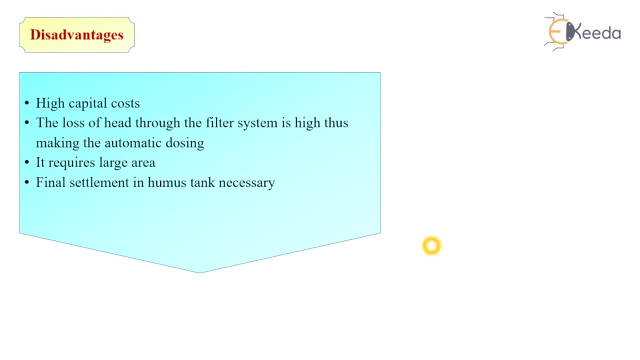 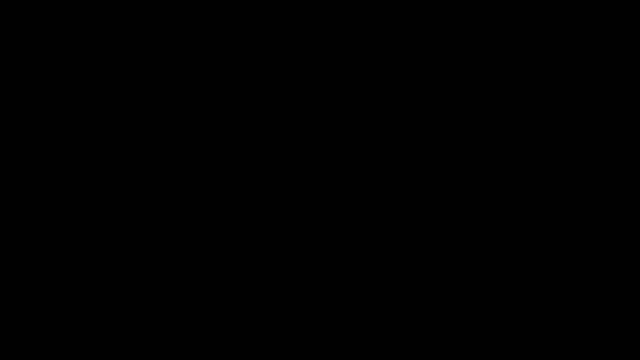 Through The Filter System Is High, Thus Making The Automatic Dosing It Requires Large Area Final Settlement In Humus Tank Necessary. This Is Part Of